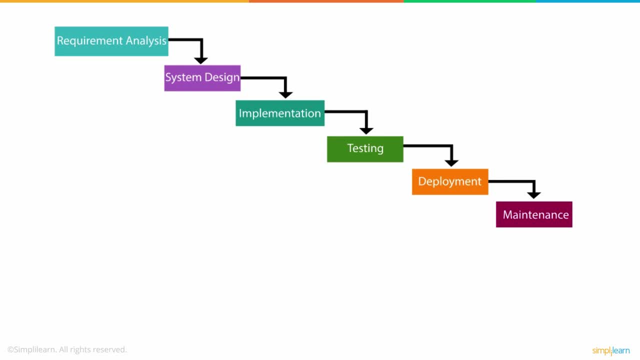 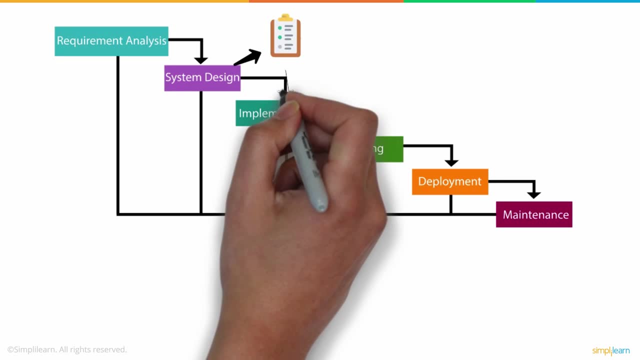 where the output of one phase acts as the input for the preceding phase. The waterfall model consists of a series of steps where each phase has specific deliverables that act as the input for the next phase, as it avoids overlapping of phases, as these phases are. 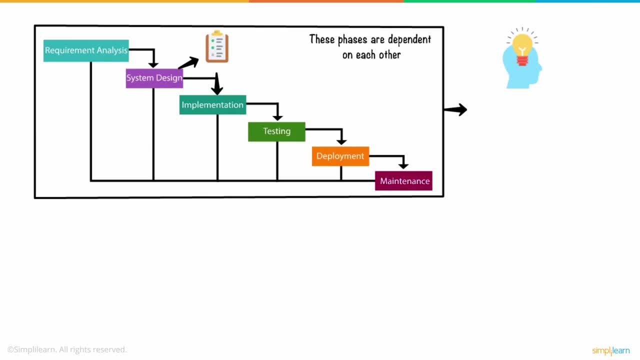 dependent on each other. This method is simple and easy to understand where prerequisites are pre-known, documented earlier and technology remains static, where there is no need for ambiguous requirements due to the delay in software delivery. In contrast, the final version is available only after completing the entire software lifecycle. 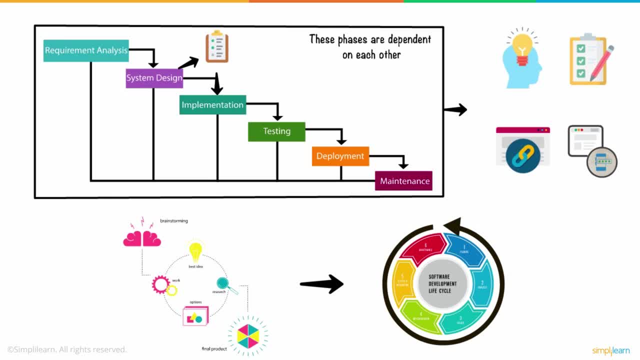 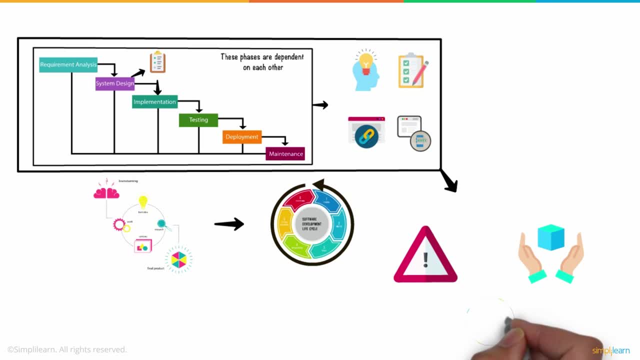 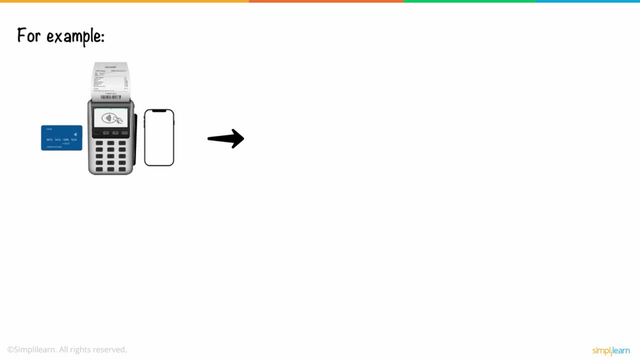 With any deviations if available. changes in the waterfall model contain high risk as changes include a new, revised version of the entire software running the entire series of steps again and again. For example, a tap and pay machine, where the machine first validates. 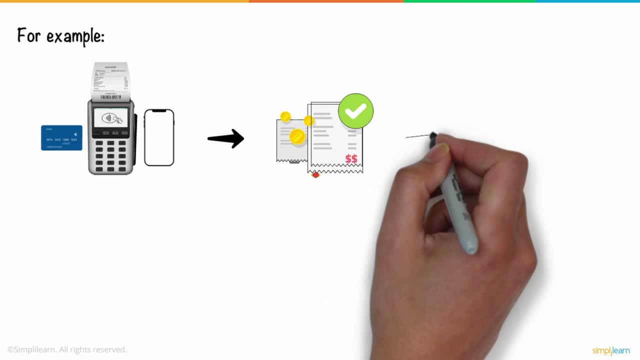 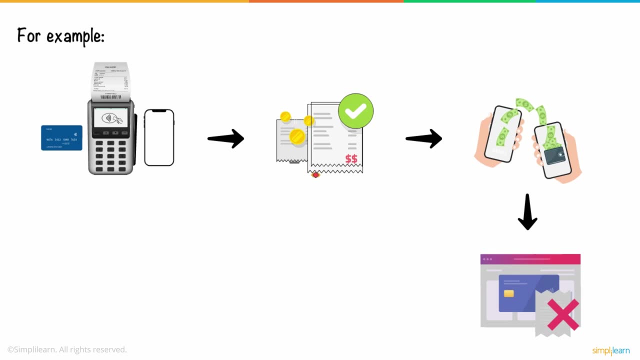 whether the customer's account is funded with sufficient funds or not, and then initiates the transaction for money transfer. Unless the validation is processed, the transaction cannot be initiated. If the transaction is processed, the transaction cannot be initiated. If the transaction is processed, the transaction cannot be initiated. 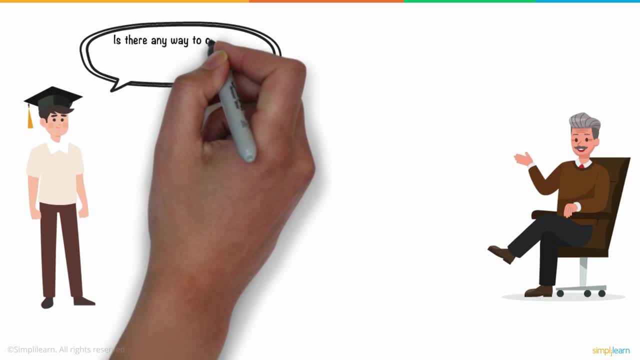 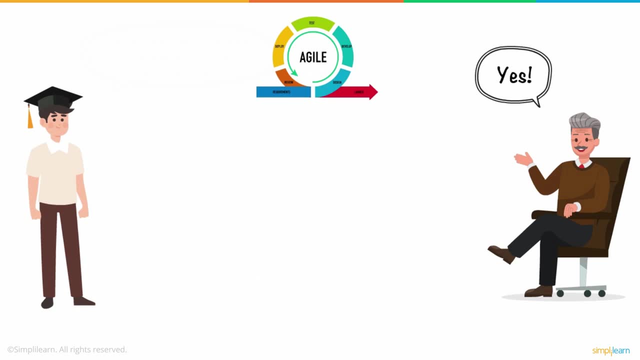 Alex was curious and asked Uncle John: is there any way to overcome the drawbacks of the waterfall model? John replies yes, Agile methodology was introduced to overcome the problems faced in the waterfall model, where Agile-based products are developed by breaking the entire product process into microservices or phases, which is faster to execute and deploy changes on the go. 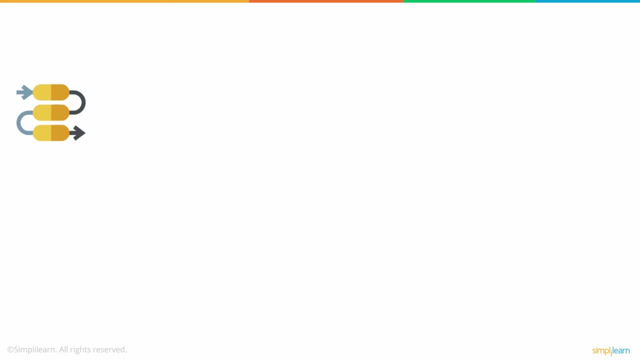 There is no need to worry about other or previous tasks while working on one particular phase. Agile-based products don't require any particular timeframe to deploy changes, unlike the waterfall model, where the whole product is treated as one single unit and each process is dependent on the preceding processes, where deploying changes leads to. 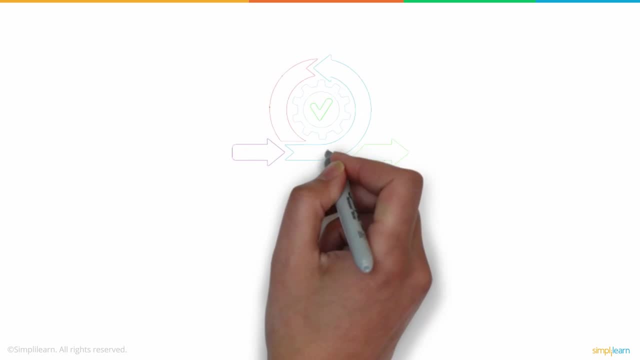 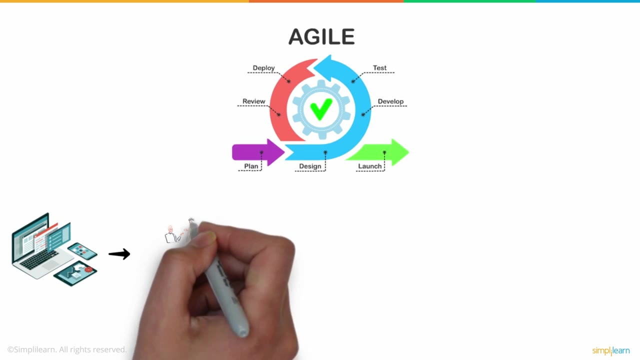 downtime. How Agile products are developed. Agile-based products are developed using the Agile lifecycle. At first, the developed product is implemented in an actual working environment for customers and stakeholders to check its deliverables and functionality. After client reviews, the official product is launched in a real-time working environment.